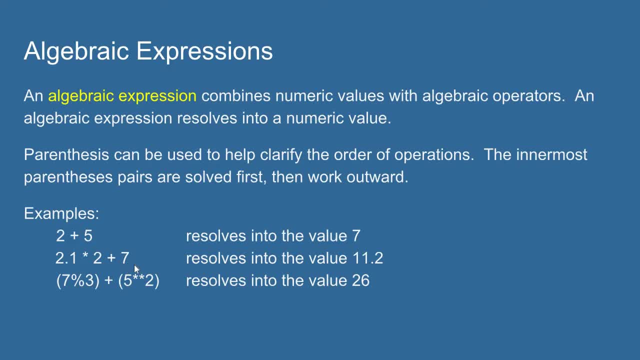 I have two point one times two plus seven. Well, the algebraic operators. in Python, they have an ordered precedence in which they follow. So for example, in Python a multiplication will always occur before an addition. So if I wanted to, so in this example, two point one times two will resolve first. 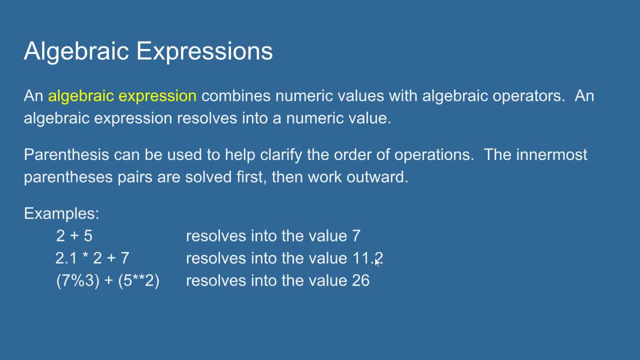 which will give me four point two. and then I'm going to add seven, which gives me eleven point two. But if you want to be clear, when you have a more complex algebraic expression you can use parentheses to help organize your expressions. When you add parentheses, the innermost parentheses. 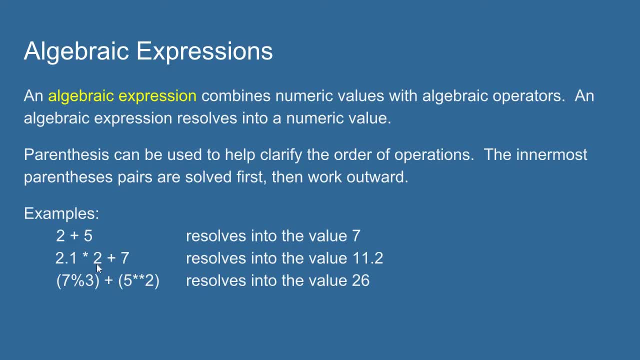 are solved first and then you work your way out. So if I wanted to add two plus seven before doing the multiplication, I could put a pair of parentheses around the two plus seven. My last example: here I have seven modulus, three plus five to the power of two, So seven modulus. 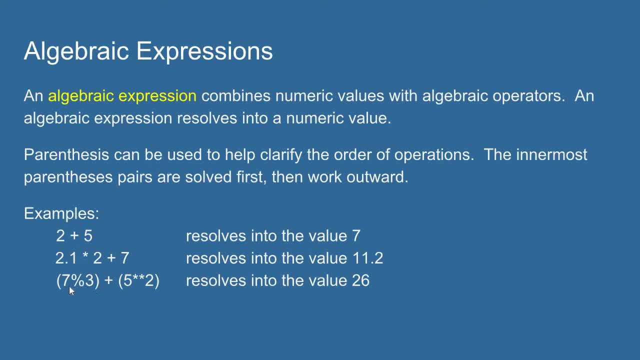 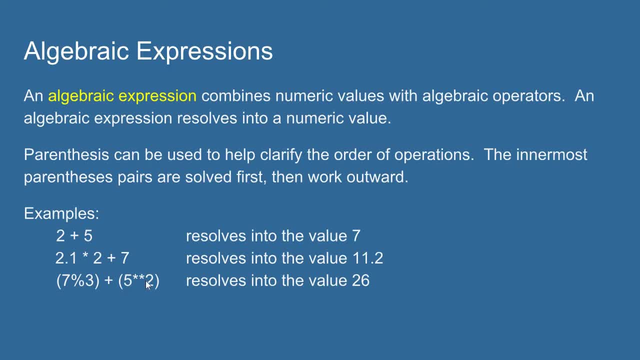 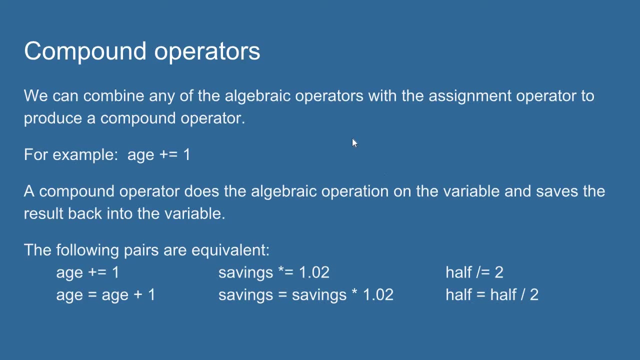 modulus gives us the remainder Five to the power of two is five. squared Five times five is 25.. 25 plus one is 26.. Now compound operators. we can use compound operators when we want to do an algebraic operation against a variable and then save that result back into the variable. It's a shortcut. 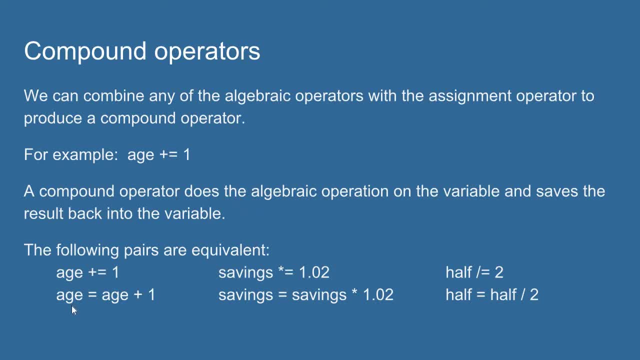 syntax here. So, for example, let's say I wanted to add one to whatever value was an age. I could just write it out. I could say: my new, my new age is equal to my old age plus one. I'm going to take the old age value, add one to it and then 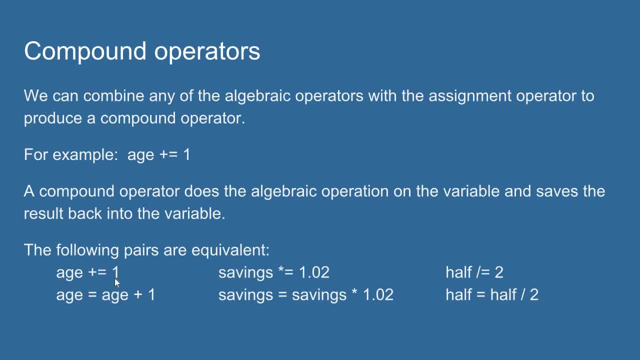 save that result back into the variable age. Well, compound operator saves me a little bit of syntax. So age plus equals one. we'll take one, add it into age or add it to the value that's currently an age, and then override. 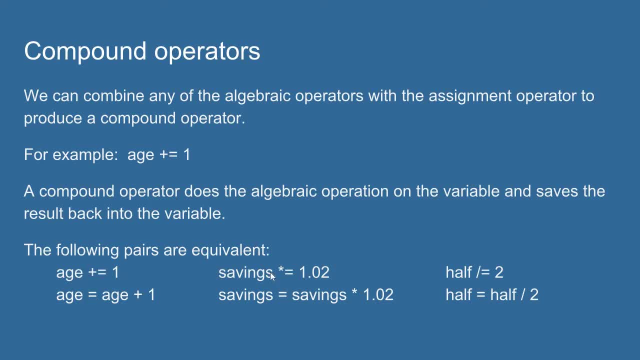 That value with the new summed value- Let's look at this one savings times equals 1.02.. I'm going to take 1.02, multiply it by whatever value is currently in savings And then I'm going to save that result back into savings. 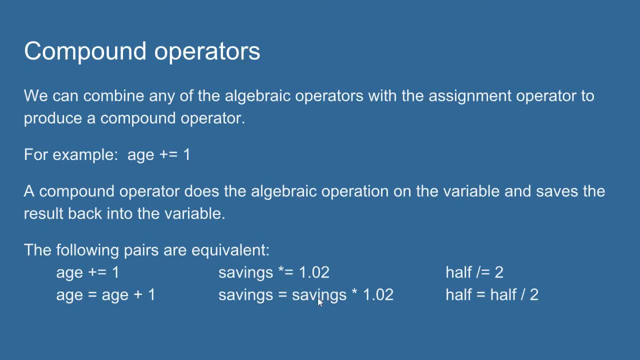 So these are equivalent. the new savings is equal to the old savings, times 1.02.. Half divided by equal to, I'm going to take the value that's currently in half. divided by two, I'll get a new value, And then then I'm going to save that new value back into the variable half. 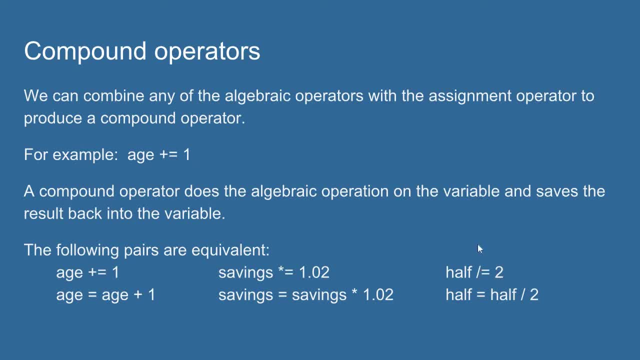 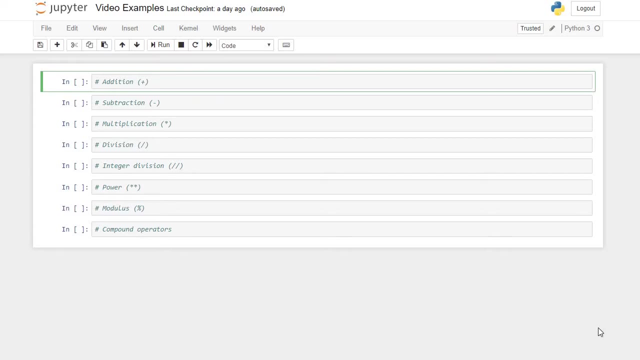 So compound operators allow you to do an operation on the value, on the value that's in the variable, and then it automatically saves that value back into the variable. Let's open up a quick little Python document and walk through a couple of these operators just to show how they work. Addition is. 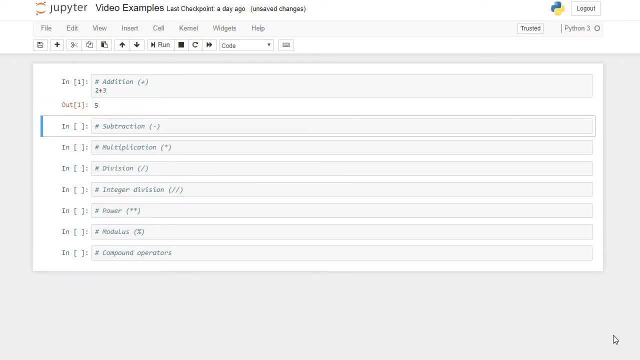 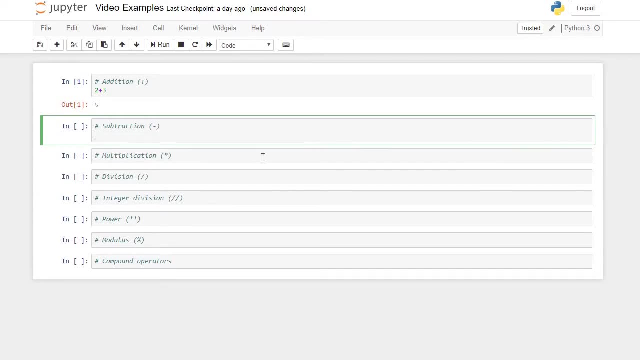 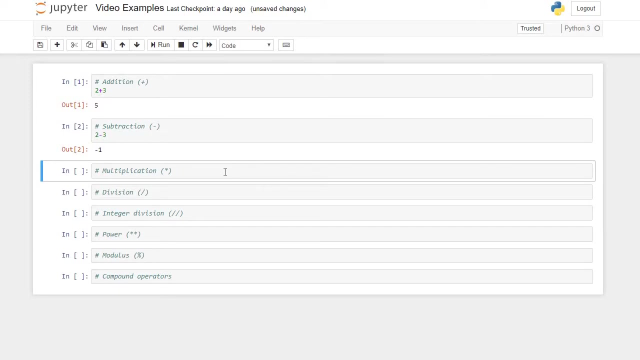 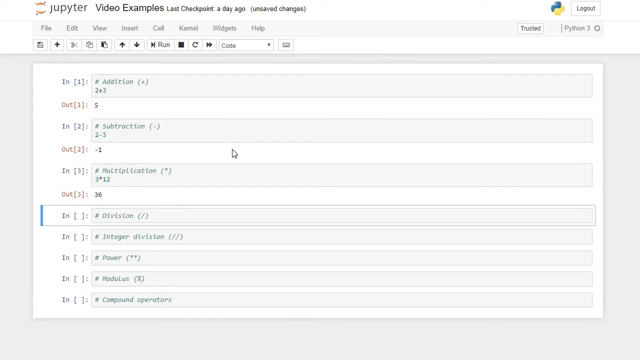 probably pretty straightforward: Two plus three gives me five, So the addition operator adds, the plus operator adds two values. So if I say two minus three, subtraction operator subtracts it. so two minus three gives me negative one Multiplication operator. So if I say what's three times 12,, we get 36.. Single asterisks is multiplication. 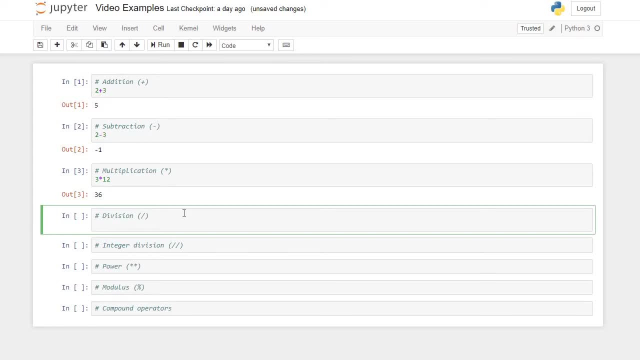 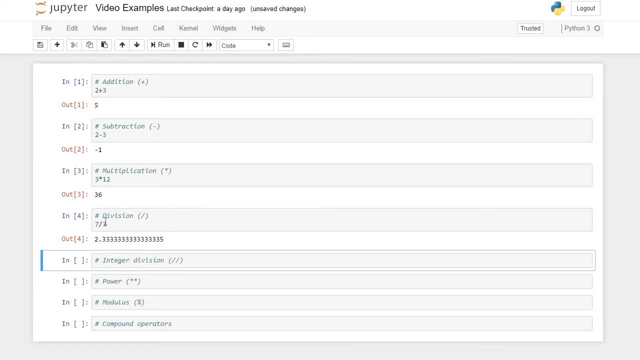 The division operator. If I say what's is seven divided by three, I get 2.333. repeating So division operator is going to produce a float value regardless of what you are multiplying or dividing. So if I said 7.1 divided by three, 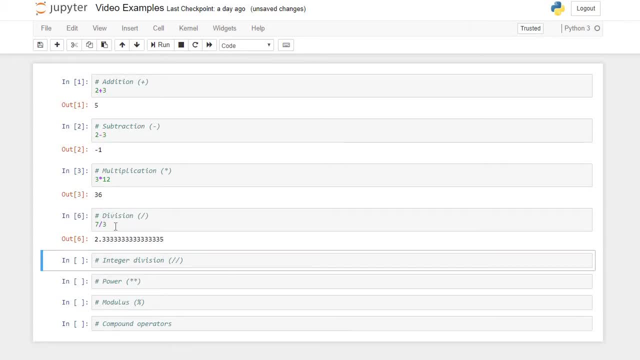 I get a float: Two integers divided by one another. I still get a float- Integer division- integer division works. the way integer division works is it's going to do the division, but it's always going to produce an integer data type. So you 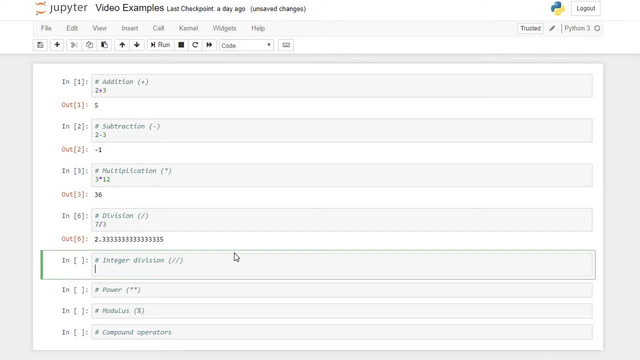 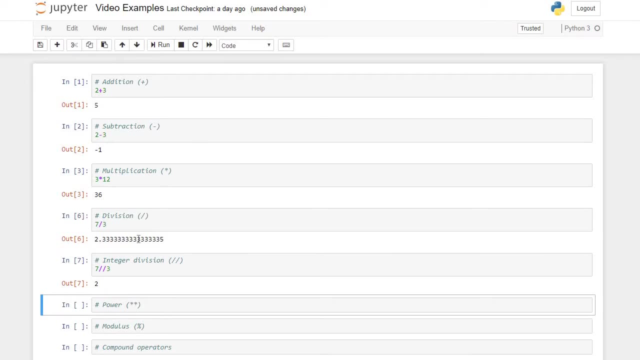 will lose the fractional portion of the division. So for example, if I said seven integer division by three, it gives me two. seven divided by three is 2.3 repeating. But when we do integer division we throw away the fractional part and we only keep the integer part. Okay. 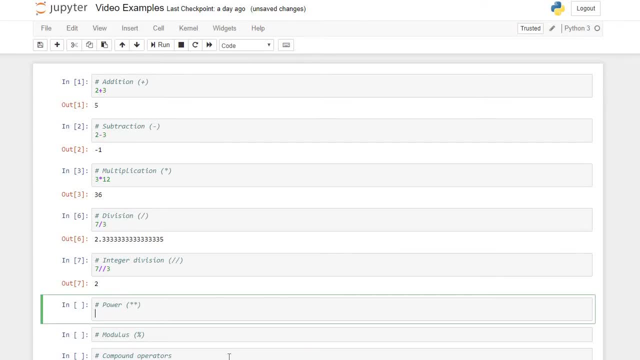 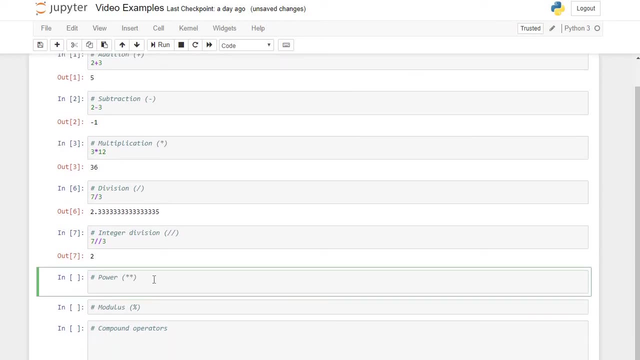 let's try again. Power power operator. let's see if I can put more space here. Power operator is if I wanted to do what. if I wanted to do what is five cubed? So, for example, you might see it written as five to the third power. Well, I could say five to the third power. 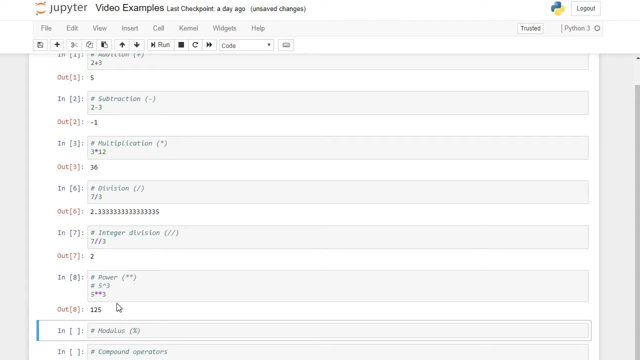 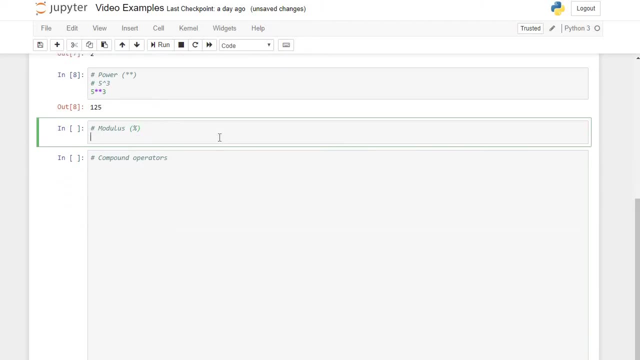 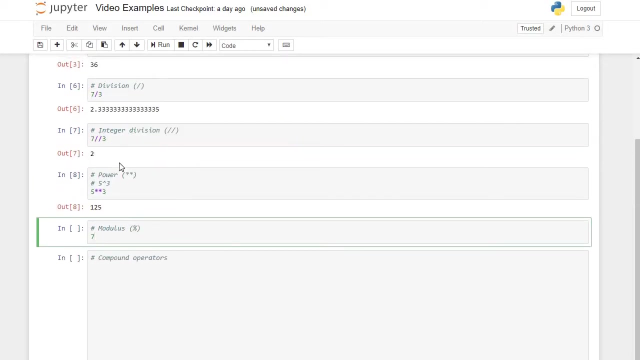 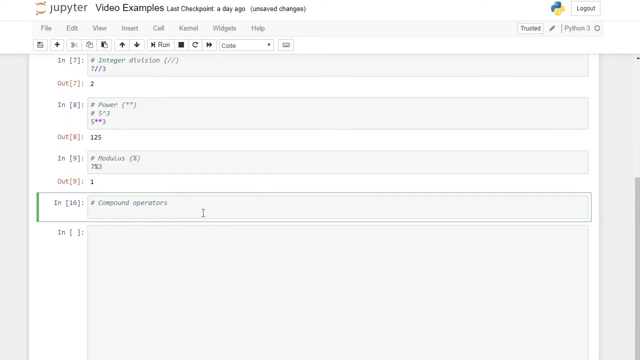 this is how we implement that in Python. So five cubed would be 125.. Alright, modulus. modulus gives me the remainder. so we did 7 divided by 7, integer division. 3 gives me 2. should be 1 left over. so 7 mod 3 gives me 1. now let's look at compound operators. the 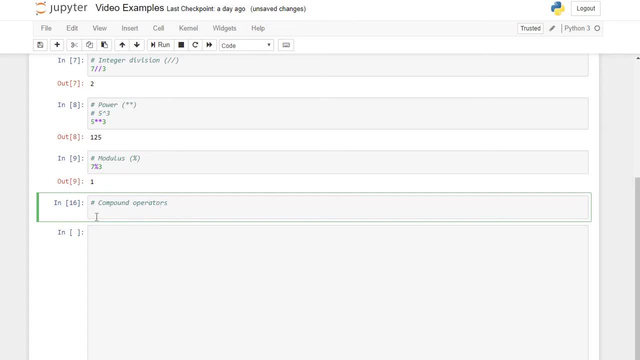 compound operator does an operation against the variable value and then saves the result back into that variable. so let's say I have the variable pow2 and I store 2 into it and I want to keep multiplying this value by 2 so I get 2. 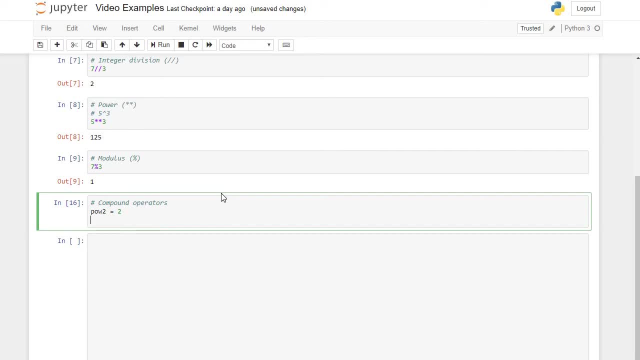 4, 8, 16, 32, all right. so what I could do is I could say: well, pow2 is equal to the old pow2 times 2, so pow2 is 2, 2 times 2 is 4. I'm going to store the value 4 back. 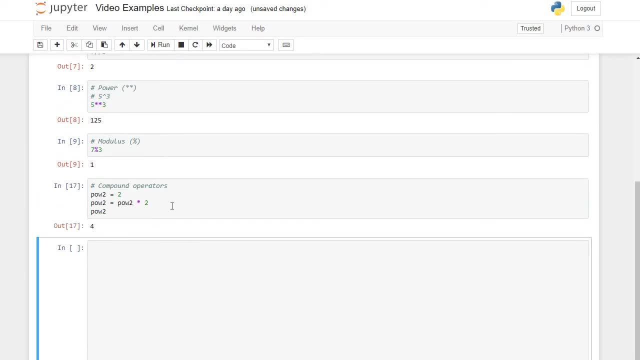 into pow2. so if I print my variable, it should say 4, and it does. but what I can also do is I can say: pow2 times equals 2. let me do that again, so I can say: pow2 times equals 2. let me do that again, so I can. 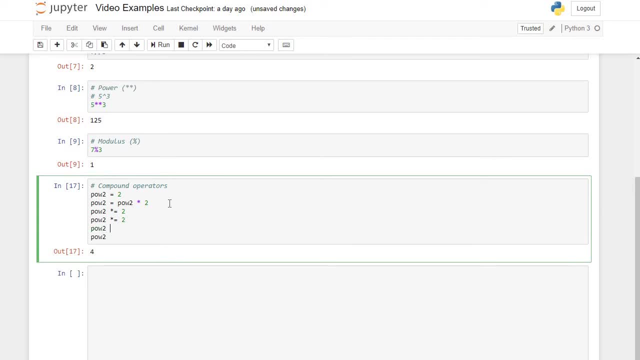 do this a couple times 2. pow2 times equals 2. so the way this compound operator works is: these two expressions are, or these two statements are, equivalent. pow2 times equals 2 is going to take whatever value currently is into, which is 4. multiply it by 2, so it's 8, and then we're going to save 8 back into. 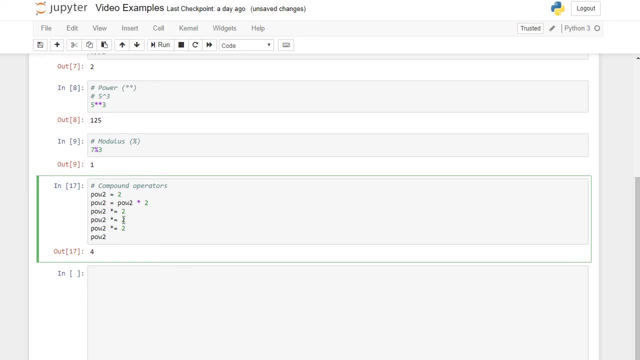 pow2. so pow2 is 8. 8 times 2 is 16. I'm going to store 16 back into pow2, so pow2 is now 16. 16 times 2 is 32. I'm going to save that result back into 32. so when I run this: